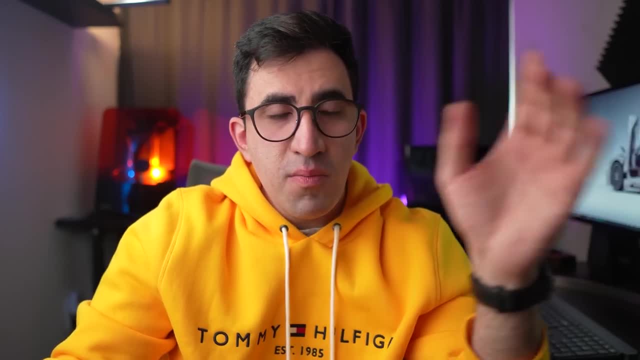 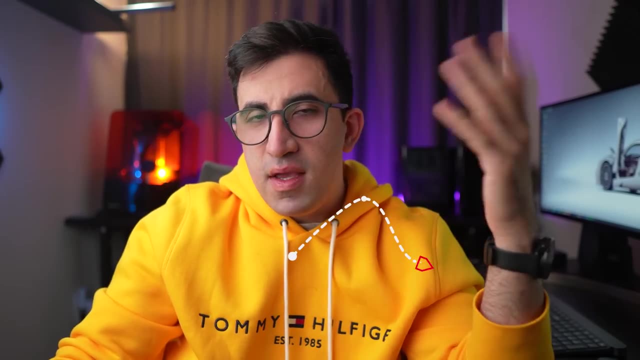 There are AI integrated with CAD to some degree, but it's not there yet. If you say AI has been taking over copywriters with this rate, the rate for replacing CAD designers is slower, and this is for various reasons. First of all, 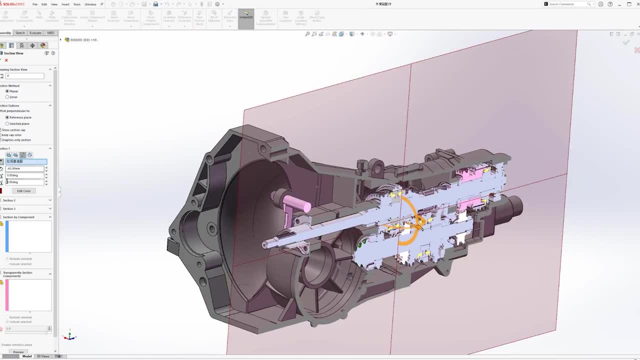 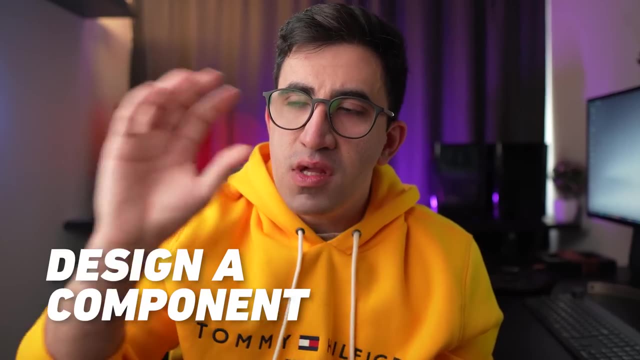 modeling a 3D component in computer is not a challenge for an AI, as long as it fully understands the objective for that. If we would like to use an AI to design a component to replace a single part in an already up and running engine, it would be challenging to define all the 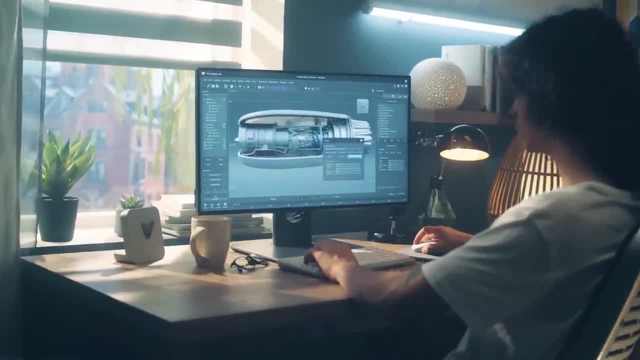 constraints and boundary constraints. It would be challenging to define all the constraints and boundary constraints and boundary constraints. It would be challenging to define all the constraints and boundary conditions of that component within that engine. Best would be to give the part to an AI and ask it to. 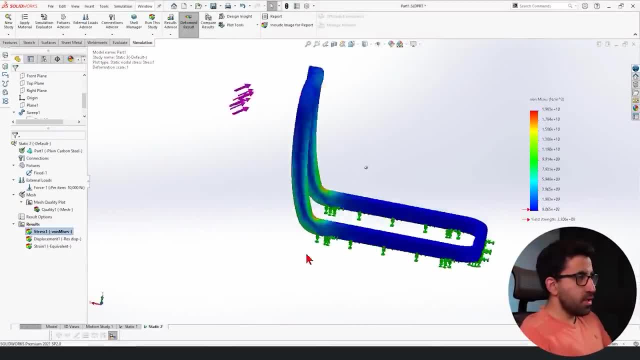 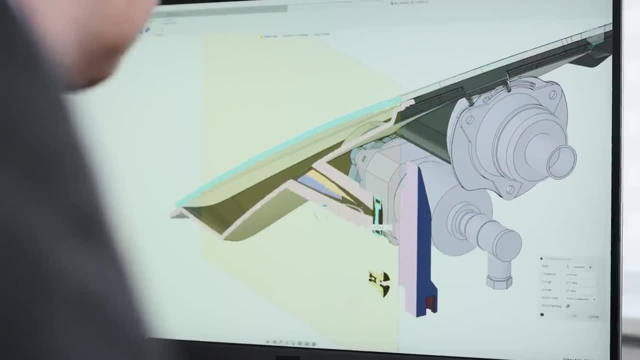 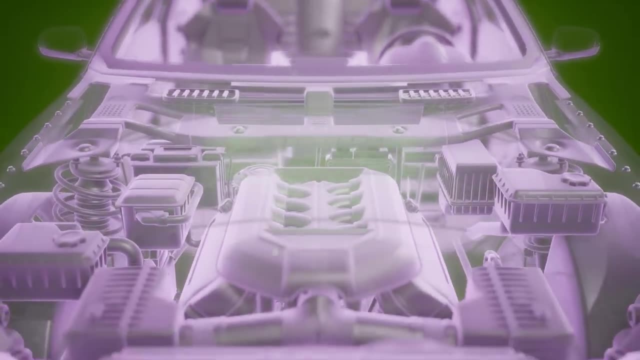 optimize it, run FEAs, optimize it. come up with a geometry out of the box that you could not have thought about, And that's a good thing, kind of like a helping tool. However, asking an AI to redesign an engine with so many horsepower, this boundary condition that fits in a BMW chassis- 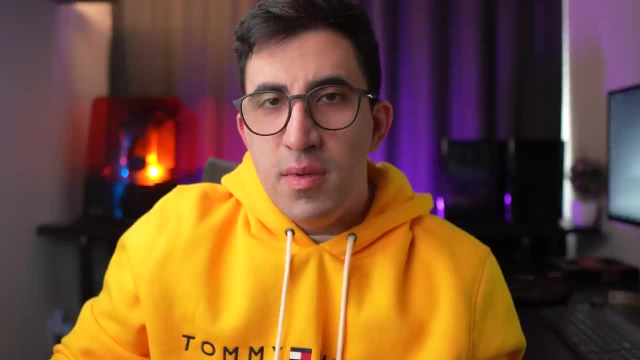 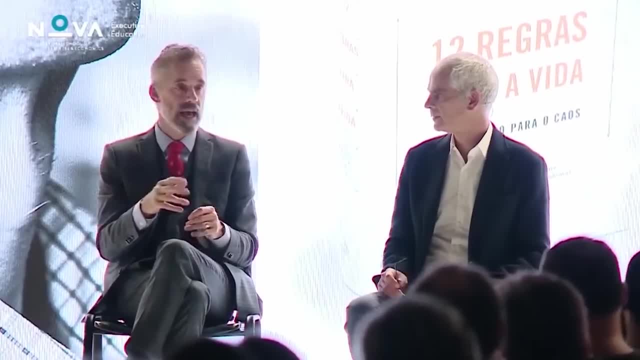 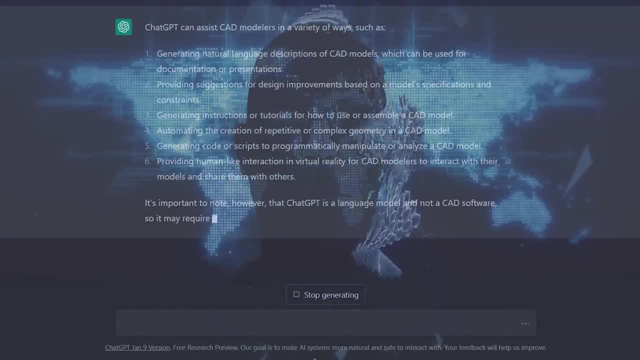 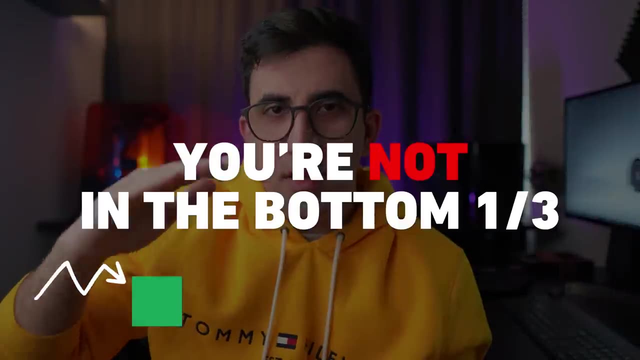 believes one third of people in every industry are going to lose their jobs, And that would be the lower one third. So, at the very very least, what you should do is to make sure that you're not in the bottom one third of CAD designers. If you know your way around and if you're good, you last. 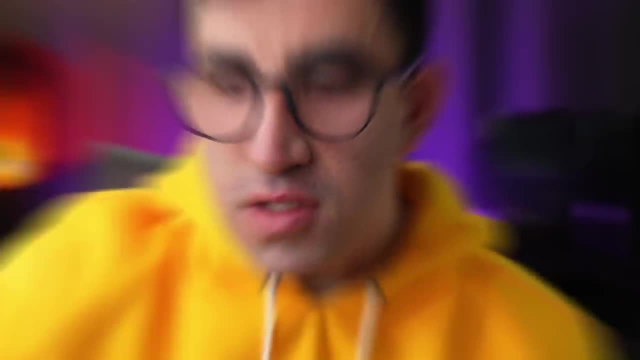 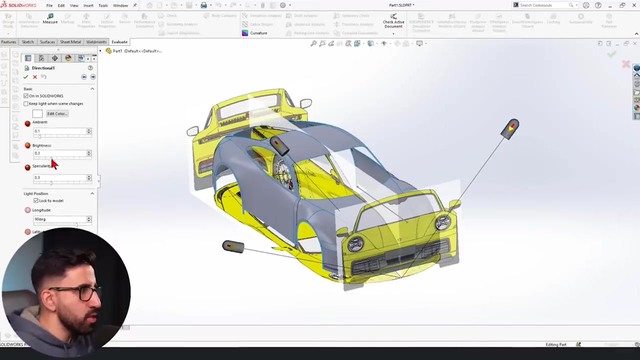 longer. However, it's nothing to be afraid of. Well, actually, Elon Musk says you have to be afraid of it. Maybe you should, maybe you should, I don't know. But I think no need to panic. all you have to do is to work on your skill and learn ai on the side. so you know. 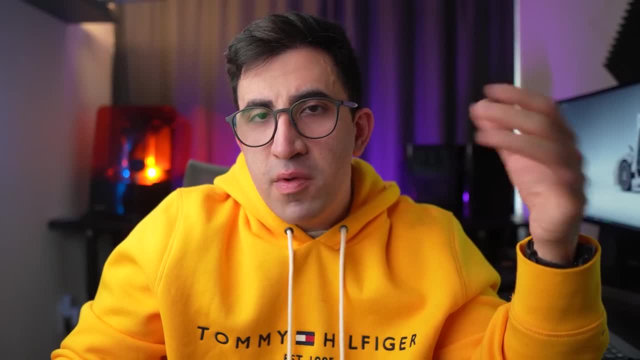 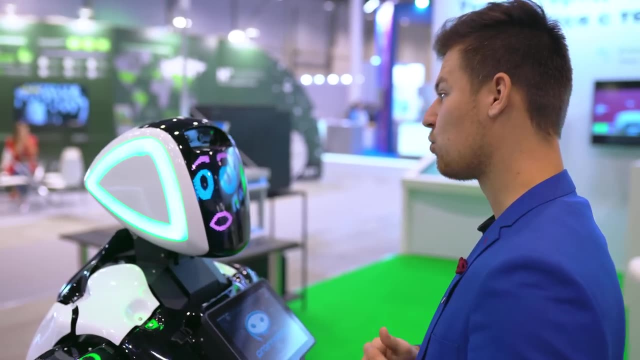 how you can take advantage of it in a world where most people are not even exposed to ai, especially people above the age of 40. just go ahead, ask your uncle, ask your aunt, ask your mom, ask your dad. see if even they have heard of chat gbt, if they work with it, if they know how to work with an ai most. 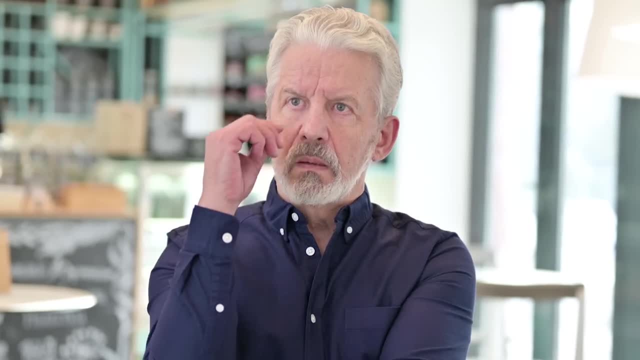 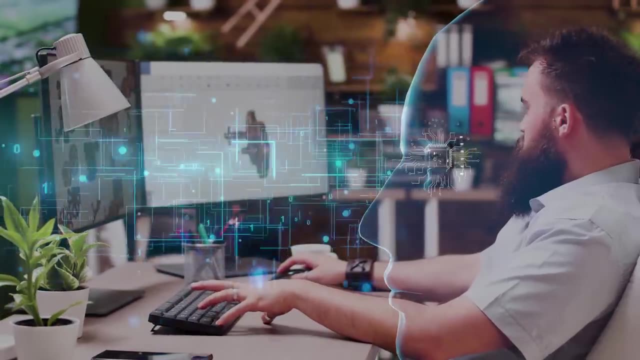 of them, don't? you are living in this world where most people cannot take advantage of this. if you are listening to this video, if you're watching this video and if you have not been taking advantage of ai, start doing so slowly. use ai, combine it with your skill and make it better. 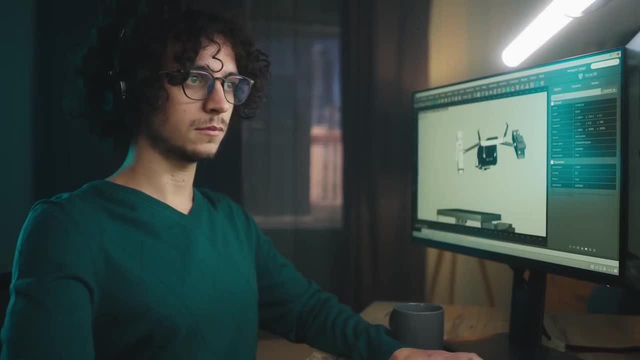 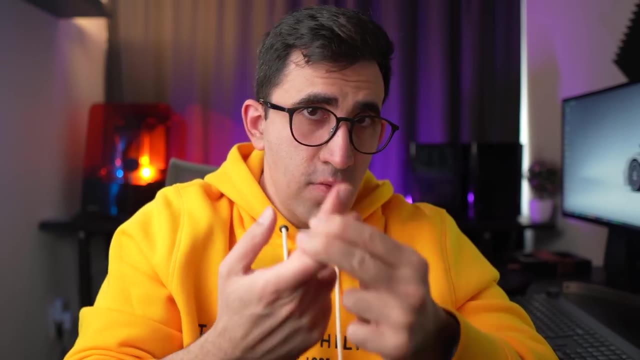 and if you do it soon, you would have an early comer advantage. not that i know what you should be doing, but you need one skill at least. you need to learn about ai as well, and you need to combine these two. however, you want to do it, do it, then let's do it. on another note, i made myself a 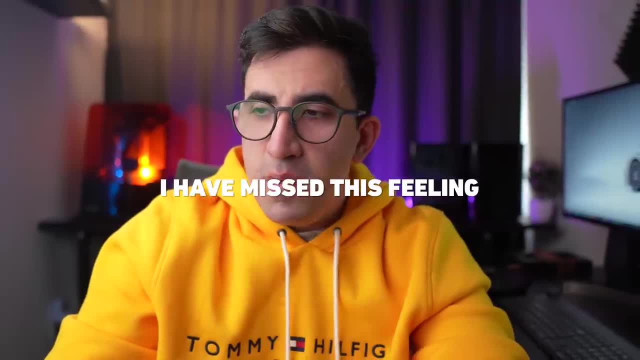 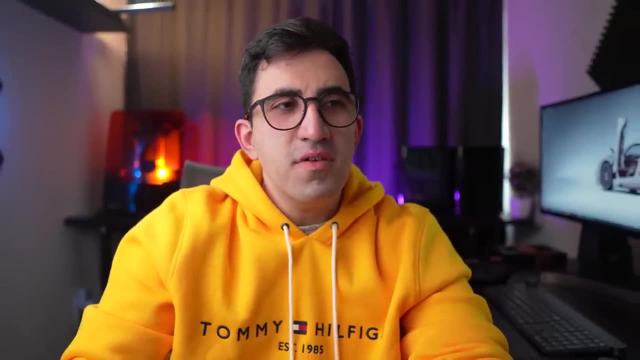 beginner again and i have missed this feeling. to be honest, i have been working with solidworks for 15, 16 years now and honestly there is no novelty in it for me. i kind of well felt a little bit cold toward it. i was not like my early days that i was. 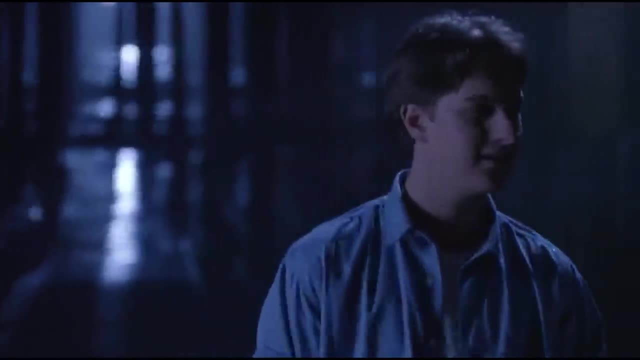 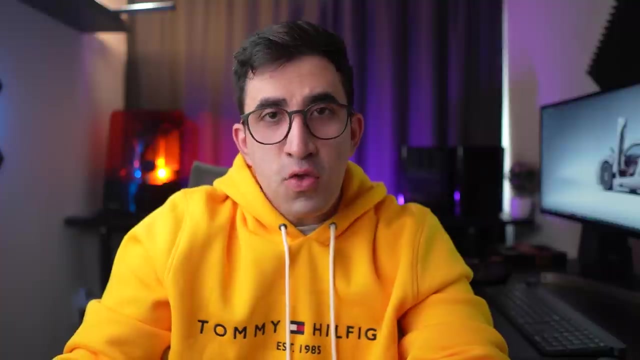 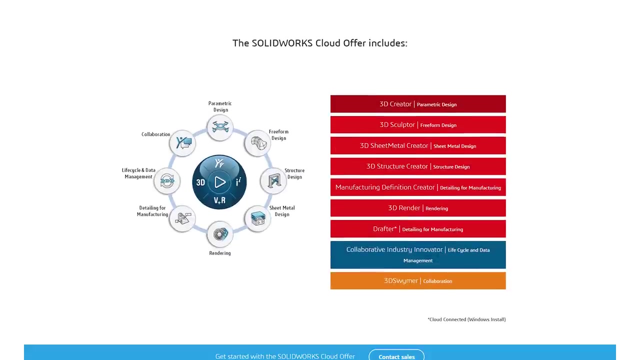 just designing all the time constantly. i mean i love it. but now i found a way to be a beginner again and feel all those excitements again. i do that by working with solidworks cloud offer, which are the sponsor of this video too. it has so many advantages, but the main. 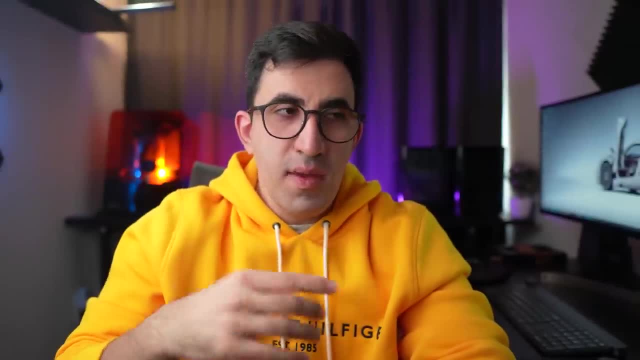 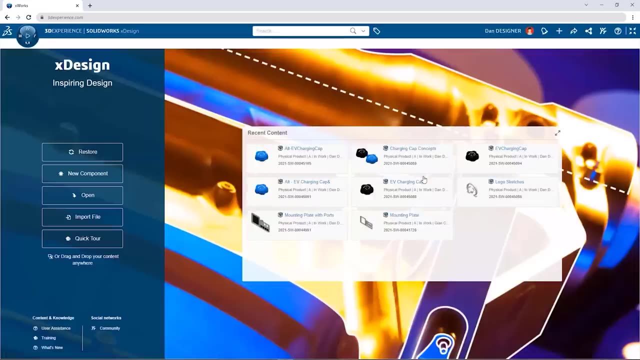 reason that attracted me to even consider working with them and even consider accepting them as a sponsor of this video is the fact that this solidworks cloud offer, which runs on a browser you don't need to download on your desktop, has a new tool called the sculptor tool x, shape and 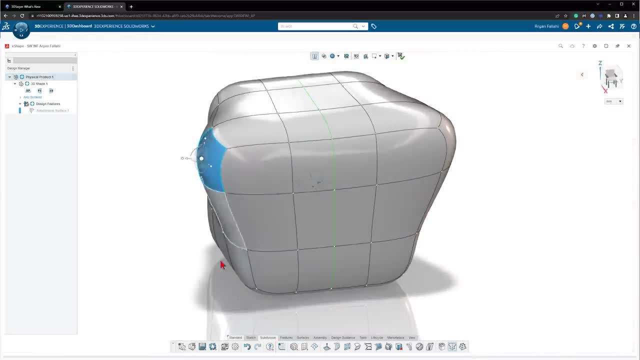 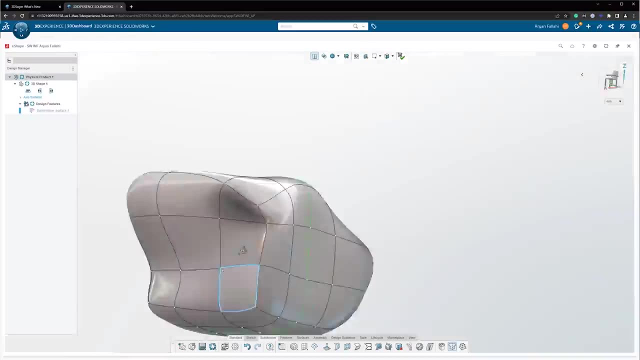 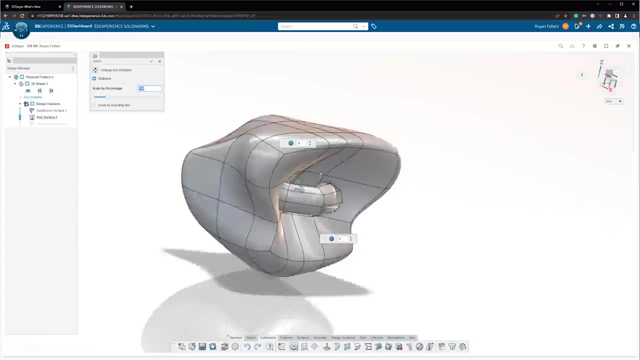 it's amazing. it allows you to just import a geometry or a surface- you know whether it's a sphere or a cube or a cylinder- and then just meshes. the component gives you the dots, edges and surfaces to just drag and form. and it's amazing. it's amazing to create organic geometries, which i couldn't have done either as easily or at all in. 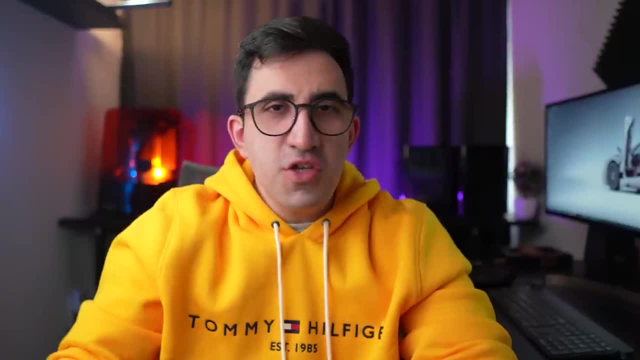 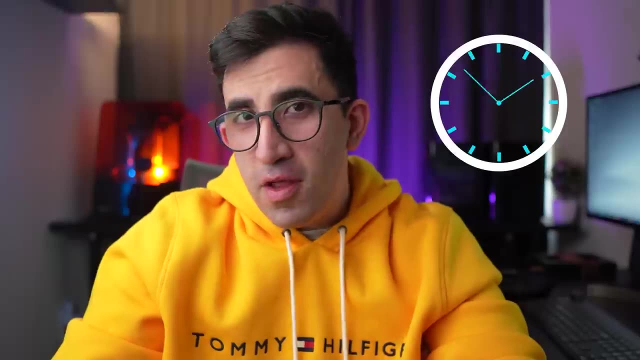 solidworks. now i feel like that motivation is back again. i have something to look up to, i have something to learn and i'm so excited i'm working with it every day for a couple of hours. i don't like going for tutorials straight away, i just want to. you know, warm up, get used to the interface a.